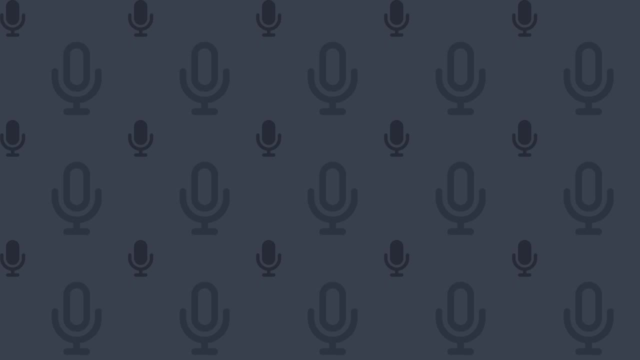 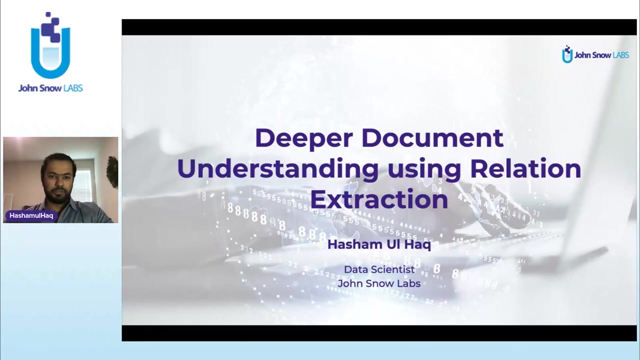 Today we will be talking about relation extraction techniques, real-world use cases and practical code implementation. We are very excited to have you here today, so, without further ado, over to you, Hashim. Hi everyone, This is Hashim, and today we'll be talking about relation extraction models. 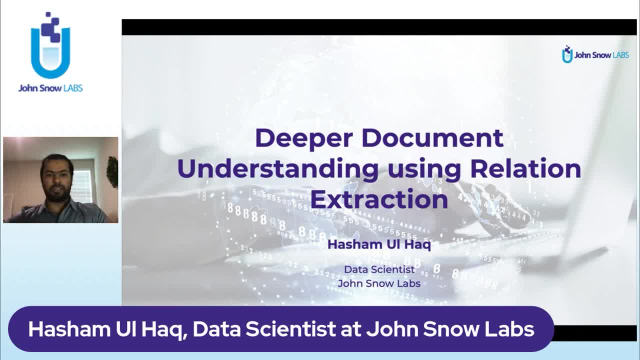 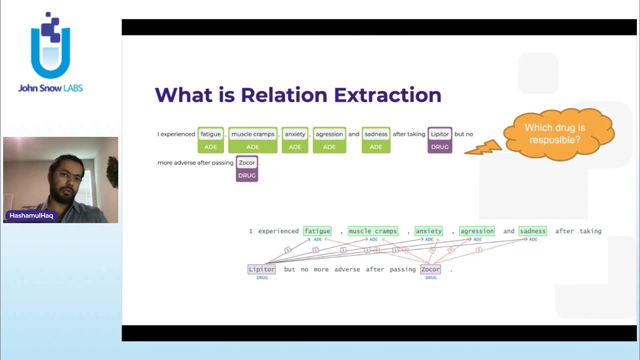 and how we use them to understand documents at scale. This is also. we have published a paper on this as well, which was published in IIII, and this is just an extension on that. What is relation extraction primarily? If you look at this screen, you would see two. 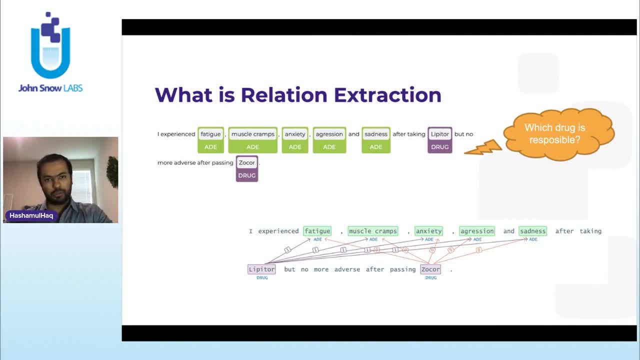 results. The first one is the NER result, which is you're feeding a raw piece of text and we try to extract entities. This is an example of adverse drug event. I've taken this example because it's pretty simple but effective. 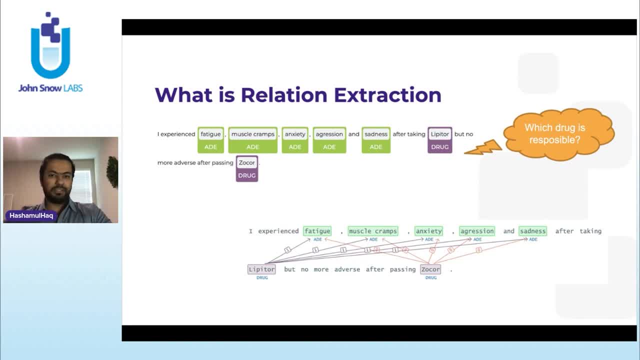 So you see that every, each and every entity is separate from each other and we get drugs and we get any adverse events, reactions, but we don't know that, which drug is responsible for which reaction, because all of these entities are disjoint. right NER model does not do. 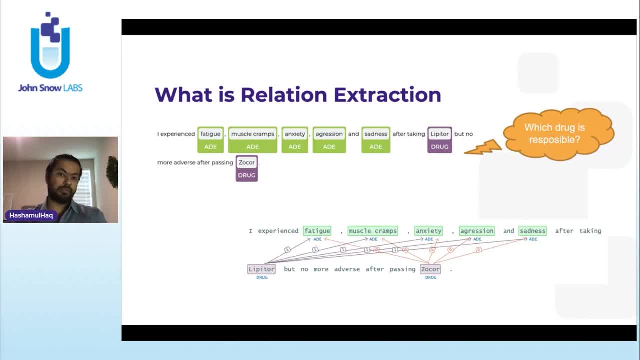 that It would only identify entities. We use relation extraction model as a layer on top of the NER model to basically reduce the number of entities that are disjoint. So that's another story of the NER model. So the question is: do we relate semantically which entities are responsible for another? 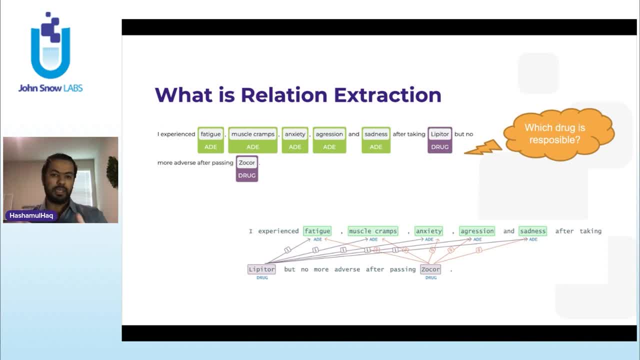 entity or how? in what form are they related? or in what form are they related In this example? it's a binary relationship. So we just say, okay, out of these drugs, which drug is responsible for which specific reaction? So, if you see the result, the second result. 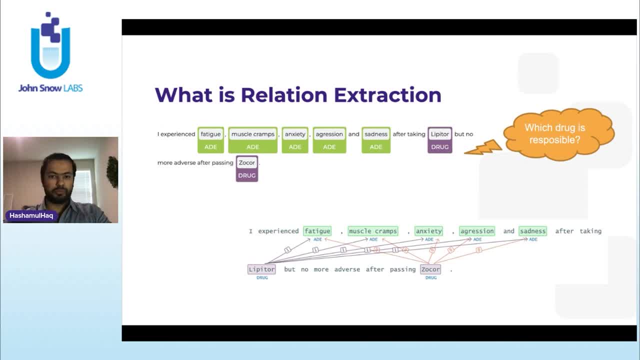 the one below it, you would notice that Zocor did not want to have drugs. Zocor did not, was not responsible for any of the reactions. so we so the model, we train the model to identify, to just say, okay, if, if the drug is responsible or it is not. it's a very binary relation model. 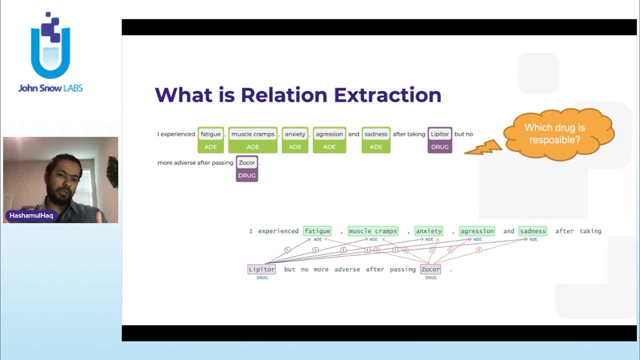 and if you look at the results, it would say that Lipitor was the one that was responsible for fatigue cramps, anxiety, aggression and sadness. but there were no after. there were no reactions or side effects after taking Zocor, so this tells. this is how we relate. so now, when we have this information, 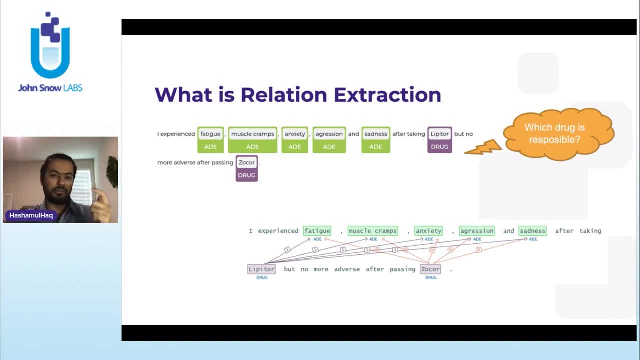 we feed in a piece of text, we now know that Lipitor was the one responsible for these reactions and not Zocor. so this is a layer on top of any our layer and which we try to semantically relate entities. now, this relationship can be of multiple types. it could be a temporal relation as well, for 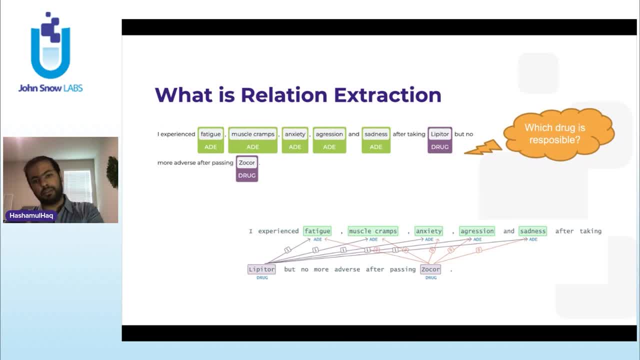 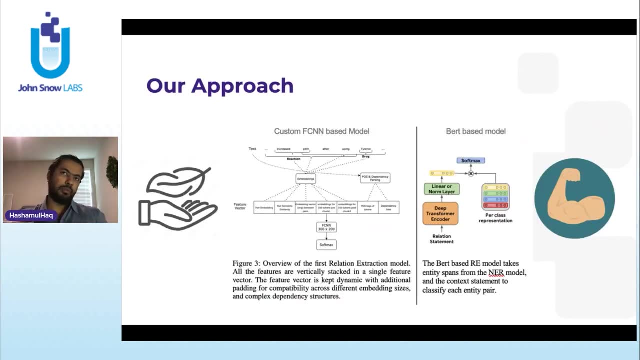 example, where we say one event happened after another event, because again event extraction would be disjoint, the entities would not have any relation until we create a relation with a, with a model. these are all deep learning models. how we go about this problem is we have to. we have developed two basically approaches. one is our custom feature. 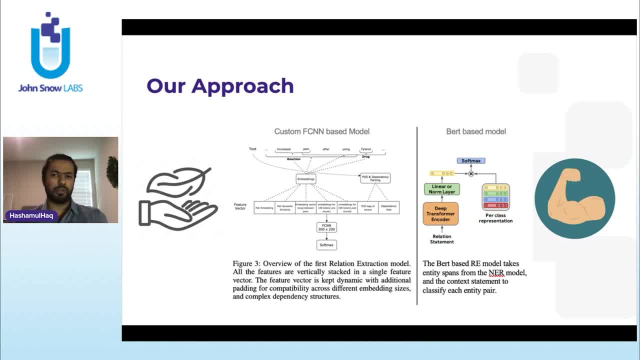 and feature engineered fully connected neural network and the other one is BERT one. so our the reason we do it two ways in is for scalability. so for simpler problems like this- adverse reactions where we have only one clap, when we have, where we have only two classes binary classification, we use the lighter model. 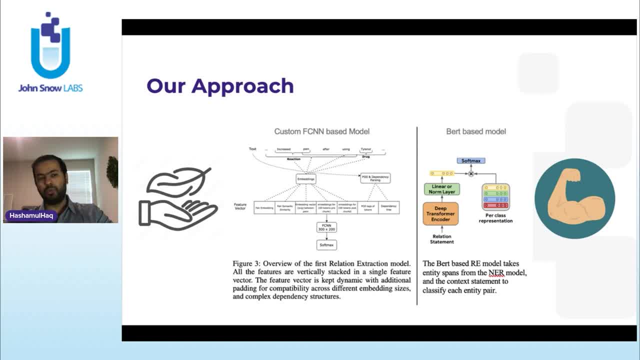 which which is basically tuned for maximum speed, and we do compromise on, you know, accuracy, but it is light and the way we designed it, we created, we tested and we created bespoke features. those features are like dependency tree of the sentence and token spans between two entities, etc. embeddings, either glove or bird based embeddings. so this is 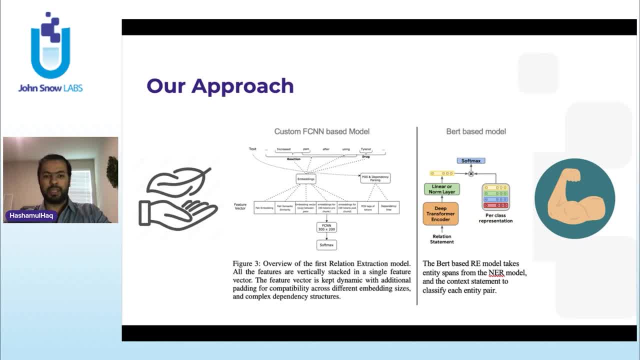 one model and the other one is the BERT one, which is an extension of one of the research papers, and in this case we we said we set the sequence length to 128 sequence tokens to limit the sequence, to basically limit our attention span, and this model is actually the best. 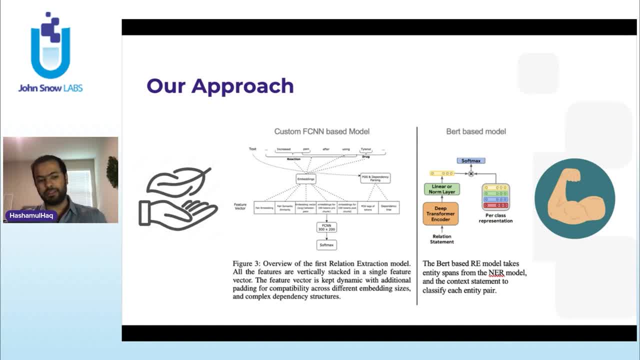 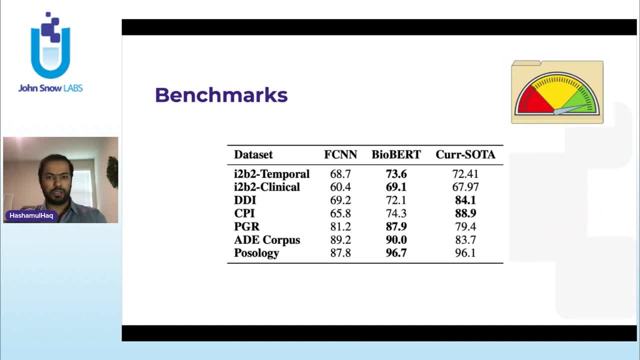 performing one, not in. I mean, we have tested this and benchmark this model on a bunch of data sets and we we get best performance with this model. I'll show you right now. so yeah, these are all seven benchmark data sets. if you- I mean the links, can this to these data sets can be provided, but I do 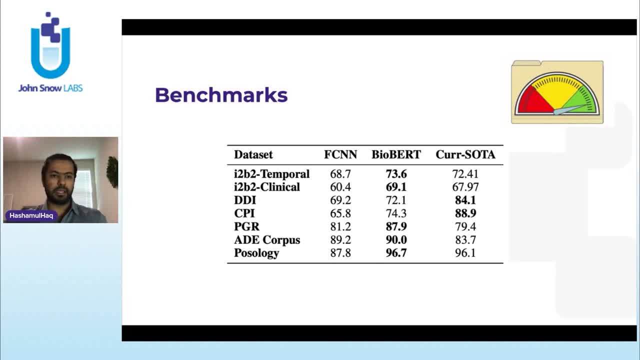 have a bunch of data sets. you know, temporal clinical DDI, drug drug interaction. you would also see here ADE and gene relations, pathology relations. these all benchmark data sets and the BioWert model that we have developed is actually better than the existing state-of-the-art models by in some 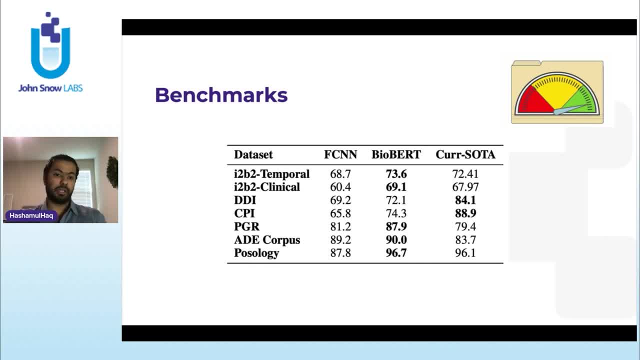 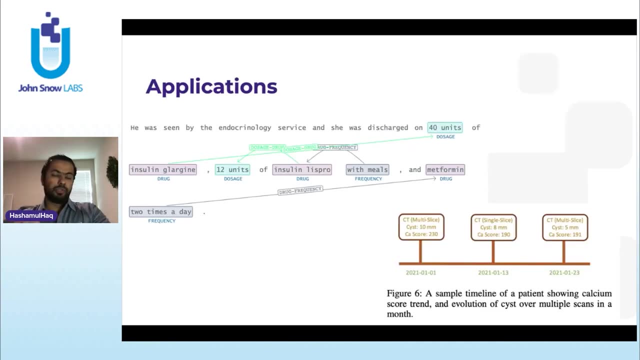 cases by just a few percentage, but in some, in the other cases, by some great margin, like the PGR model and, yeah, the ADE model, our BioWert model is state-of-the-art as for now. so now that we've discussed that, we have we know how- to the importance of basically relation 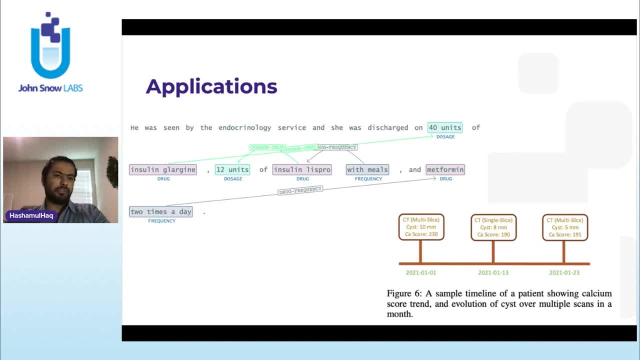 extraction on top of NER. what are the applications? these applications- one one that I've already shown you that I mean- extract drugs or and they and link them to their reactions. so in raw piece of text you would know which drug is responsible for which reaction. but it's not just related to that. for example, this is a: 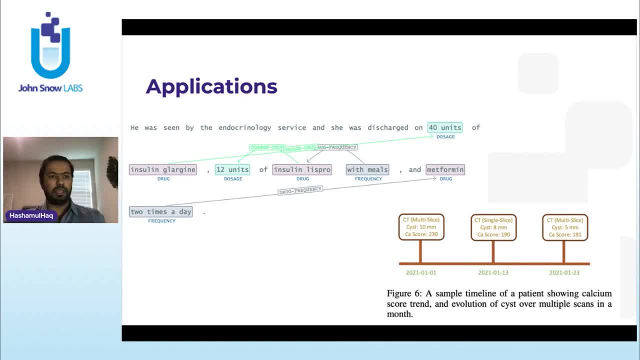 prescription or discharge node of a patient. so in this case it's: uh, we, we. when we do relation extraction, you would see that now we're relating dosage and drugs and their frequencies and either form- you know what form- oral or any other form. so this is, if you look at this example, uh, it was seen. 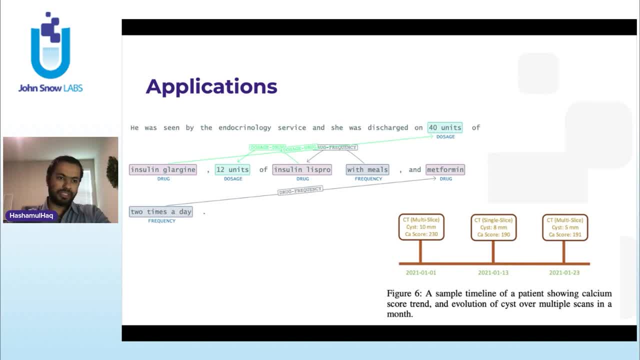 by discharge in 40 units of insulin, and so this insulin has is of 40 units, but the other type of insulin, its dosage is 12 units and the frequency is with meals. and then metformin is two times a day. the benefit of this is we get to we get more granularity. if I were to simply extract this: 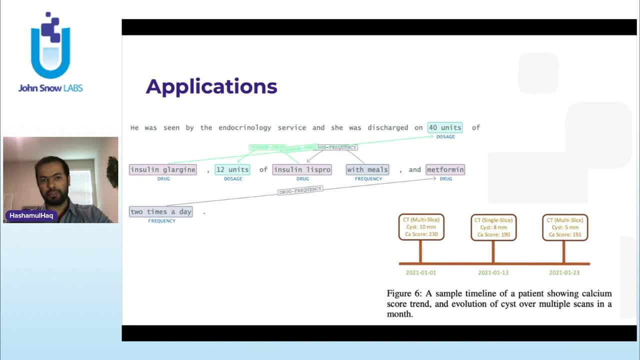 entire piece of chunk, let's say 12 units of insulin Lispro with meals. I would have to divide that chunk down and see which exact drug was prescribed in which way. but now I have more granular chunks, more precise chunks, and we link them to get a structured output. this is one application of parsing prescriptions. 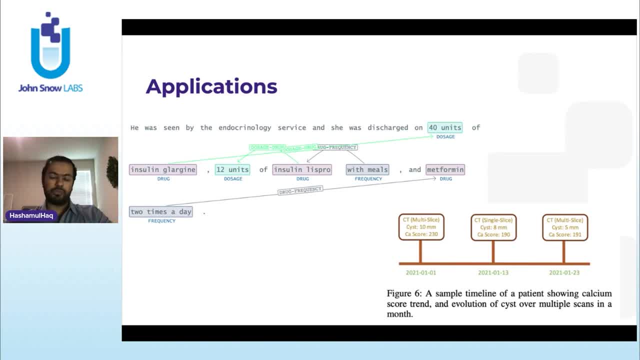 discharge summaries, Etc and other application is because now we have relations, we can identify dates and link them to certain lab results procedures. that's the second example and that allows us to get to put us to put the entire timeline of a patient on chart. so for 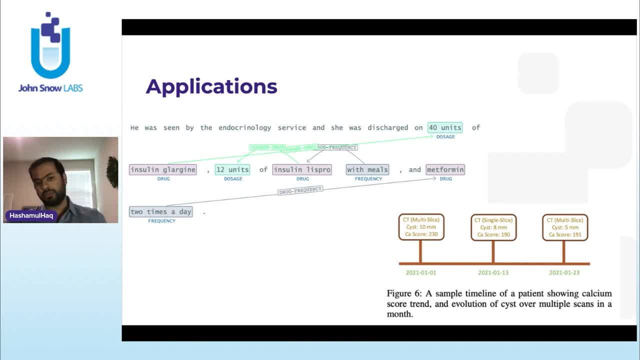 example, in this case, if there were multiple summaries of a patient over one admission, and we would process each and every report, we would extract dates for each and every one of them and we would extract test results, for example calcium score in this case and the problem in that. 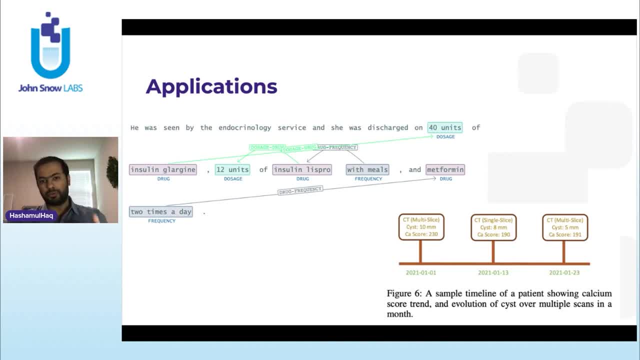 patient was. let's assist them. considering so on 2021. this was the result on, sorry, on First Jan. then on 13th Jan the result changed based on new tests, Etc, and on 23rd Jan the results got changed again and we can, we can. 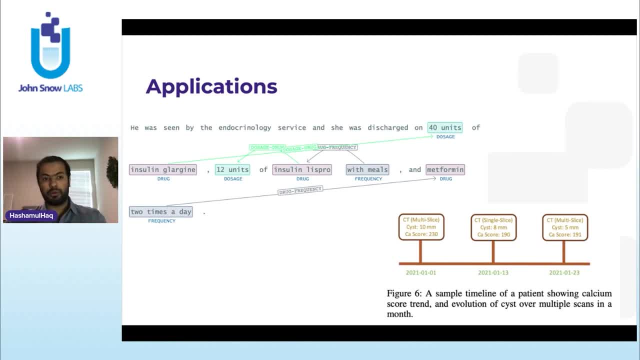 then deduce whether it's there's any improvement or any action needs to be taken. but essentially what we've done is collected multiple reports and an on a timeline, just because we can now relate entities, We can find dates, We can find procedures and we can say, okay, this date, this procedure was performed on this date. This helps us do this. 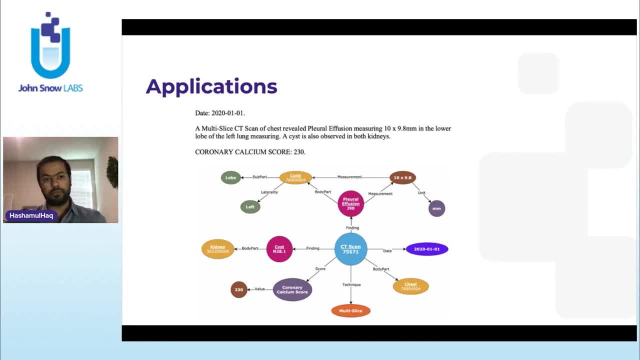 Another example of this, another application that is actually a real world project, is processing full-fledged reports and generating knowledge graphs. So yeah, everybody, we talk a lot about knowledge graphs, but what we don't realize is knowledge graphs without relations is nothing. Relations play the most pivotal or most important role while generating a knowledge. 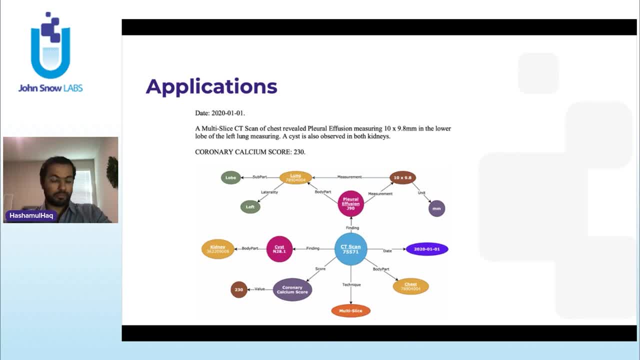 graph And this is the evidence actually. So, for example, we have a piece of a report- in this case it's a radiology report- And, by the way, this example is where all of these things come together and you get a single knowledge graph. In this we will see dates linking procedures, linking body parts. 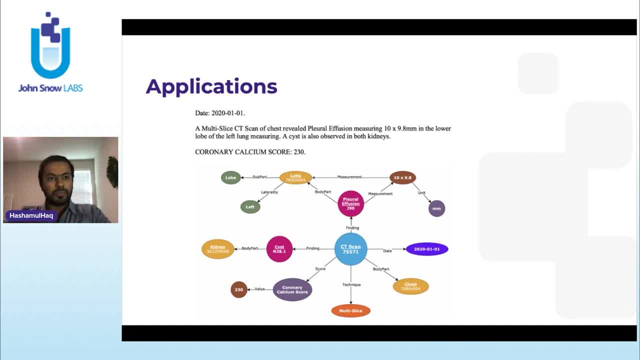 linking all that kind of stuff. So if you look at this example in this radiology report, we would see, okay, we have first Janice, the date, and CT scan was performed. but the technique of that CT scan was multi-slice. And where was CT scan performed? On chest, And what was its finding? 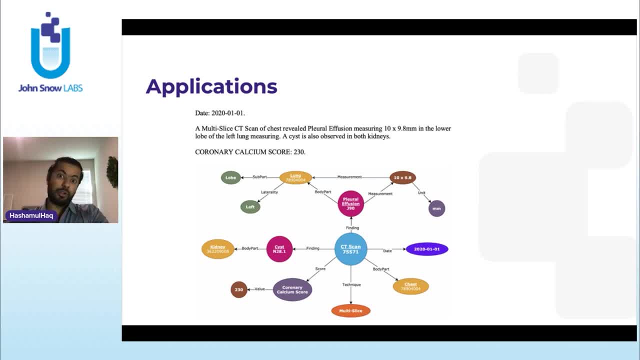 Clear fusion. And what was the measurement of clear fusion? It's 10 cross 9.8 in the lower lobe of the left lung. So the body part is lung and its laterality is left and its sub body part or subsection is low. And then another cyst was. 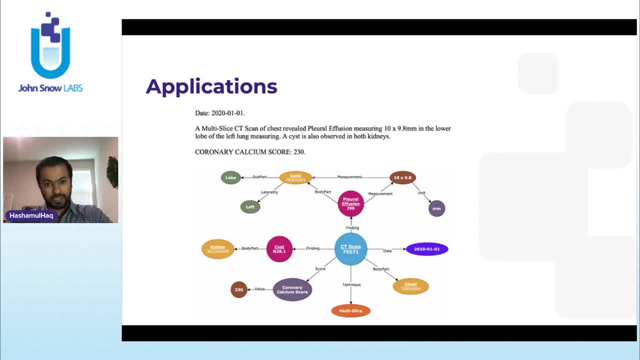 observed in both kidneys. So if you put all of this in a graph like this, you would see that the primary procedure, which is which is in the center, the CT scan, this is the primary procedure. now we link them. we link this procedure to findings. In this case, we have two basic 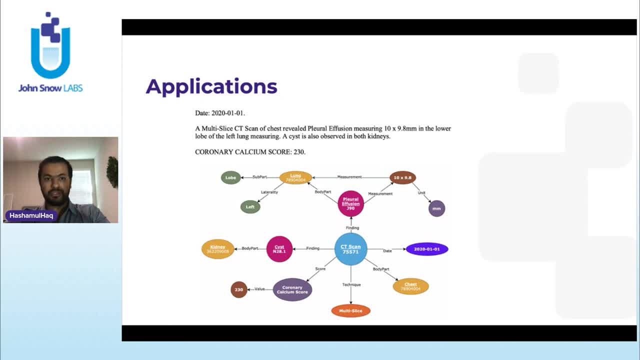 findings: One is clear fusion, The other is cysts, which is the second sentence. If we take the first finding, clear fusion, we would now link the measurement with it and the unit of the measurement, So 10, 9.8, and then we have the location of the pre-revision body part. Now 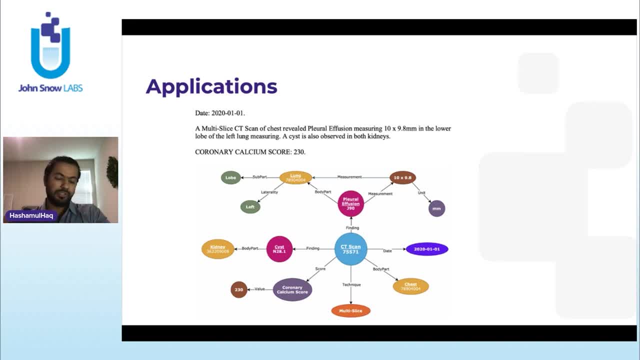 how do we know this relationship type as well? It's not just relationship, it's the unique relationship, it's the relationship type as well. we know that because now we have two different entity types: lung is a body part and pre-refusion is a finding. so the relationship between them is finding and 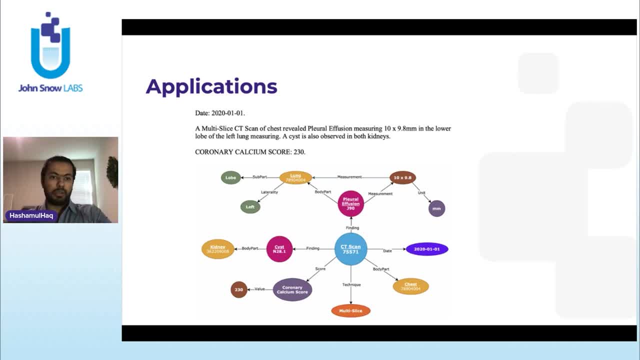 body part, so we know the type as well, and then we have sub body parts and laterality lobe and left left lobe of the lung. so this is how you would see that we create a hierarchy, with just deciding on how to create relations, and this is the power of relations. we're not simply saying that. cd scan. 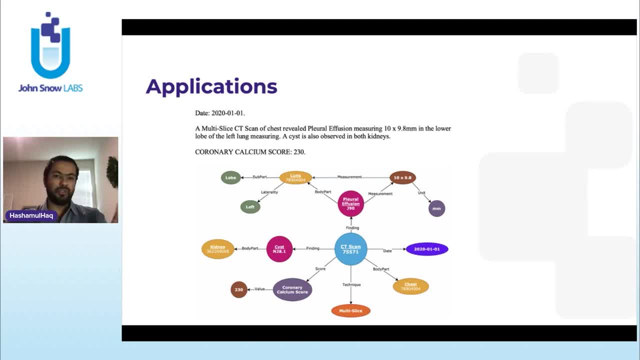 was performed on a chest and pre-refusion and the finding in the lung was this: no, we're going very, very detailed now that there was pre-refusion in the lung in left lobe and its measurement was. similarly, a cyst was observed in kidney. so this is the power of relations. 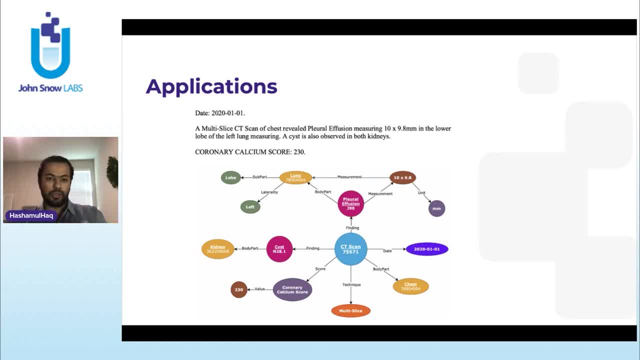 and we now have the data as well. We also say, okay, the technique of this was multi-slice and we have coronary calcium score which is 230.. The primary body part was chest. You see that we have multiple body parts. but 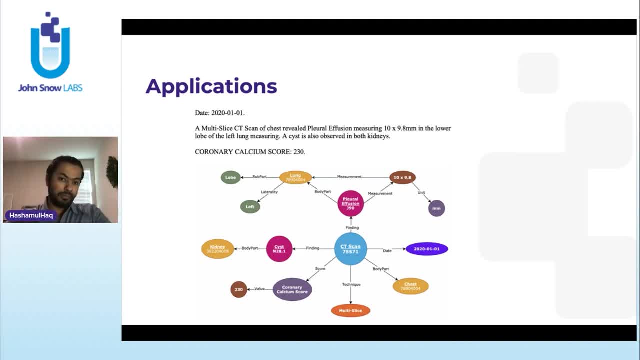 this is where I'm coming at. We have multiple body parts, but the primary body part on which CD was performed was chest. The findings of piller fusion was not in chest but rather in lung. Now this is up to the relation extraction model to decide which exact body part is linked to which. 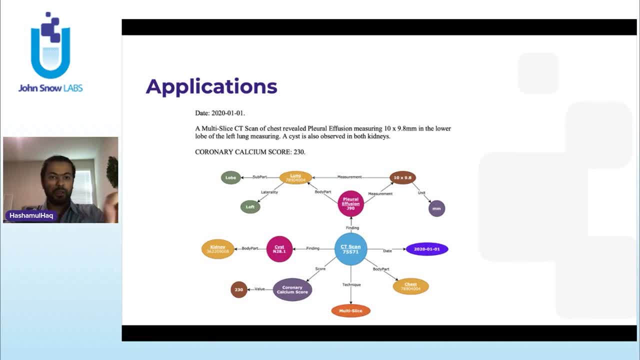 finding or procedure. So this is how we create a knowledge graph. at the end This is, if you to convert this into a JSON, you would get a completely structured data. So the magic in this is you feed in an unstructured piece of text, a large report, and at the end you get complete. 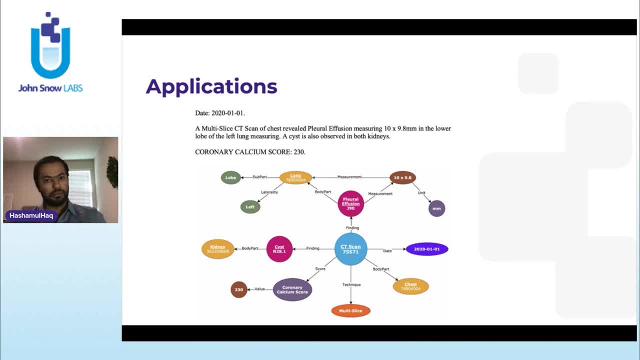 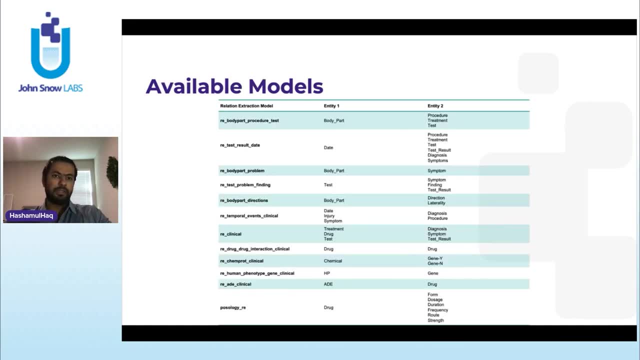 structured data With a hierarchy, So you can do a bunch of analysis, take decisions et cetera. In SPARC NLP we have multiple models for relation extraction. Like I said earlier, I showed you already RE underscore ADE, which is the adverse drug one, but we have a bunch of them And every model is 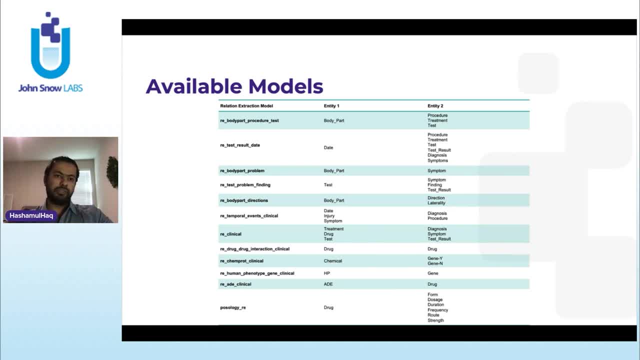 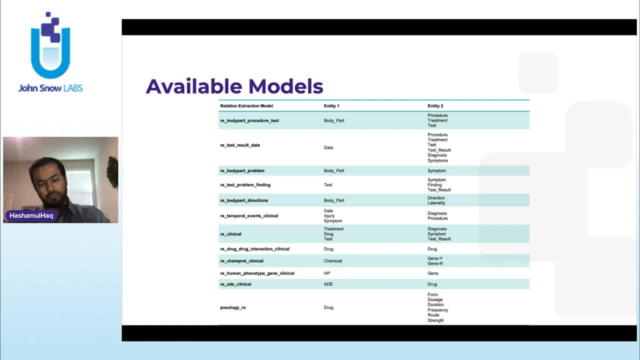 entity pairs are the entity pairs. So the entity pairs are the entity pairs. So let's say that in the case of ADE, we divide one model by two. The second model is called the second one is called the overlapped model. I hope you can see that. That is why the with different models in the 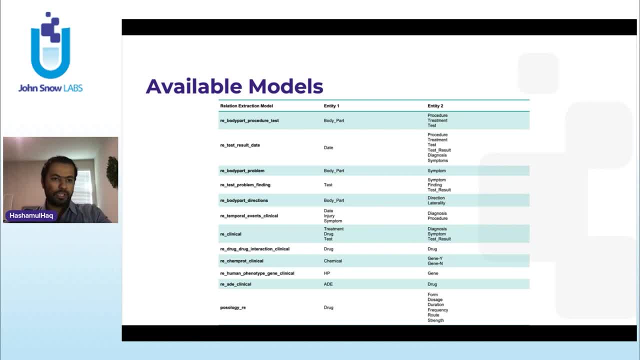 model And we end up with. till now we have roughly 10 or more than 10 models. For example, the body part procedure test would tell you relations between body part and the procedure, just like what we saw in the previous slide, CT and chest. The test result date would be: 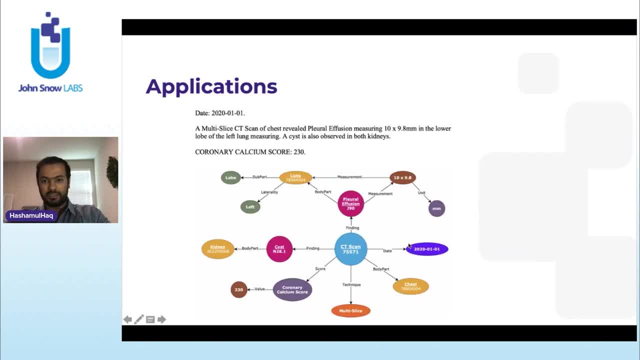 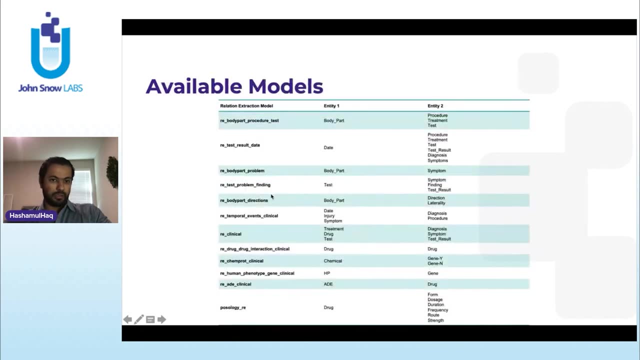 for example, if we say here, then this is the test and this is the date. If there's any results, we could also link that to date. So this would be that model would do that Body part problem, just like body part procedure. body part problem is this: lung and perfusion. 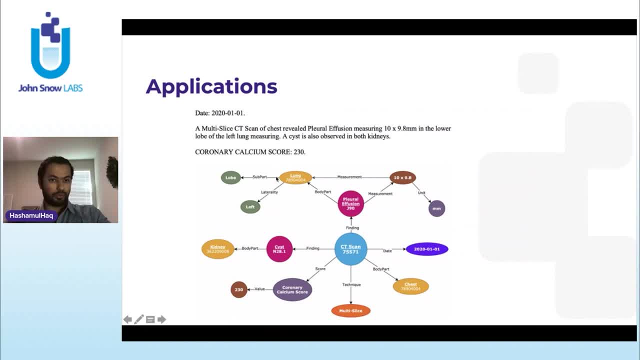 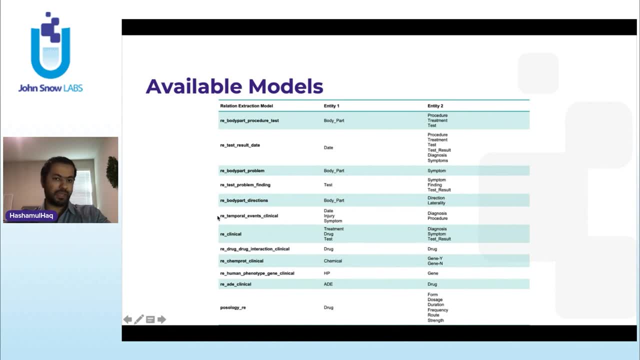 Body part directions: lung, lower left lobe. This is the model for that, And then we have some. these are binary classification models. Then we have some multi-classification models as well, Like in the case of RE underscore clinical. it would not only tell you if the 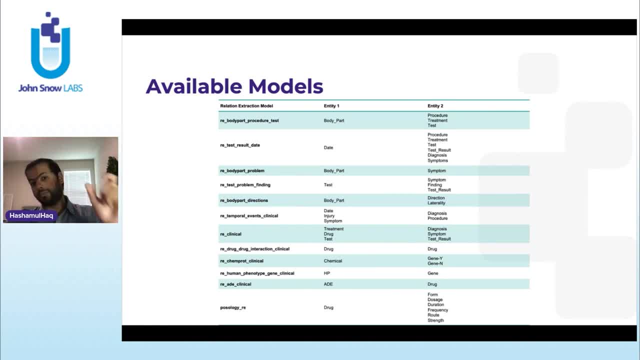 drug or a diagnosis is related, but it would also tell you if a treatment has cured a symptom or it has aggravated a symptom. So in this case we have roughly seven different classes and we get results based on the two entities, So test and test result, and drug and symptoms. 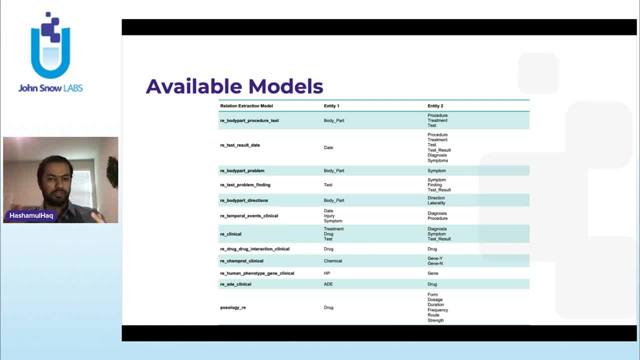 So we can say, okay, this drug cured a symptom or not. So instead of binary we now have multiple classes over here. Then we also have models for G, For relating genes, chemical proteins, et cetera. And the last one, the very powerful. 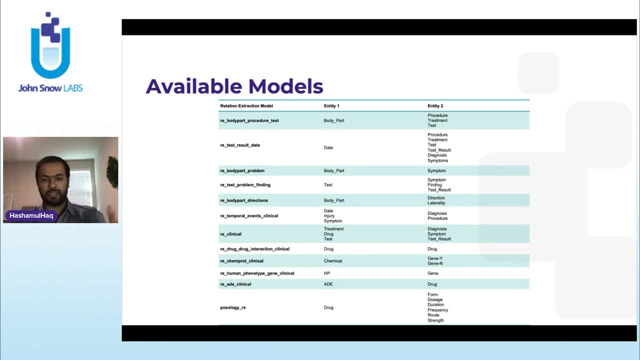 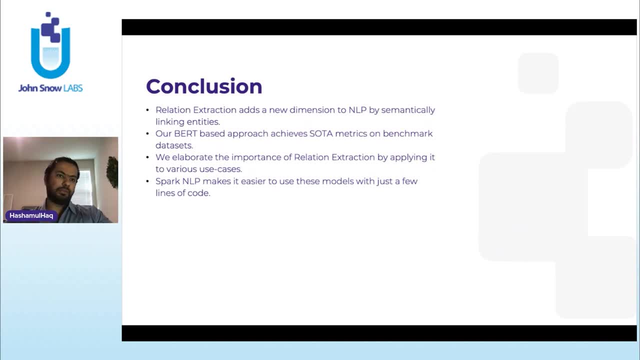 model is the pathology one relating drug and all of its things: form, dosage, et cetera. So in this talk, what we have, what we try to, the main point of this and the main motivation behind this, is only relying on relation on an named entity. recognition models would. 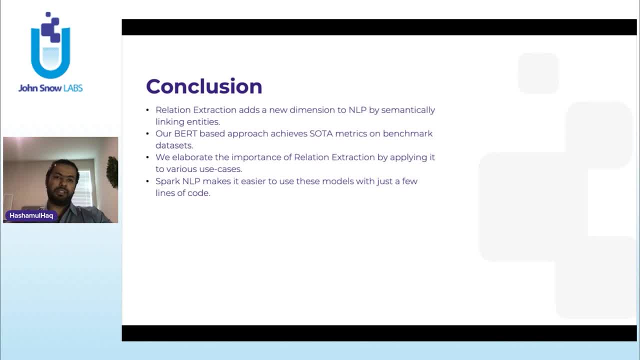 would be. basically, it doesn't allow us to go into details and extract or link entities, which is important. as we've seen, We simply simple disjoint entities. They're good for analysis, but they don't get. they don't portray the full picture for for which we 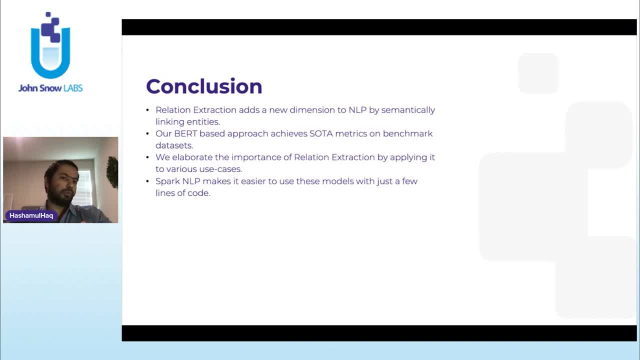 have. we have developed basically two different models, out of which the bird one is actually the soda, And we have also seen the importance and use cases, Okay, of extracting of these relations right. We're able to generate knowledge graphs. We are even. let me go back and show you one other thing. 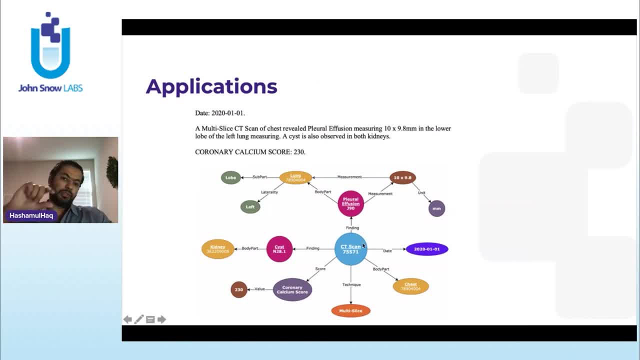 So there is one interesting use cases and that is when you try to resolve these codes to these symptoms and procedures, to codes. So if I only try to resolve cdscan, I would get a very general code. When I say code, I'm talking about CPT or ICD codes. 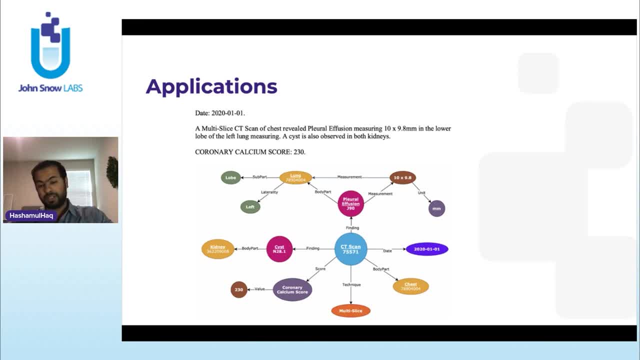 In the case of cdscan it would be a CVD code. But if I say cdscan of chest then I should get a more precise code, just like cyst of kidney. If I just say cyst, the code would be of cyst, unspecified. 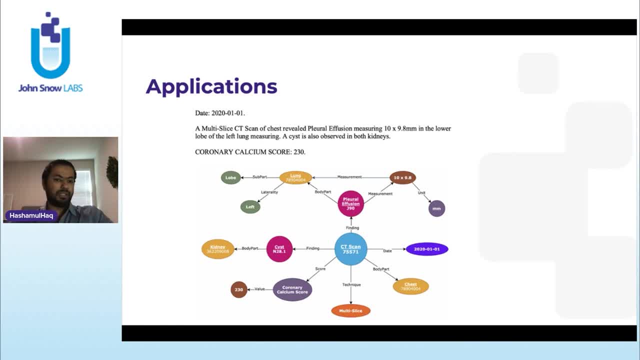 That's no good value to me, because the cyst happened in the kidney. So relating these two entities now allows me to get a more precise code, because now I know that in the hierarchy cyst has a body part- kidney- and I can generate a more enriched chunk. 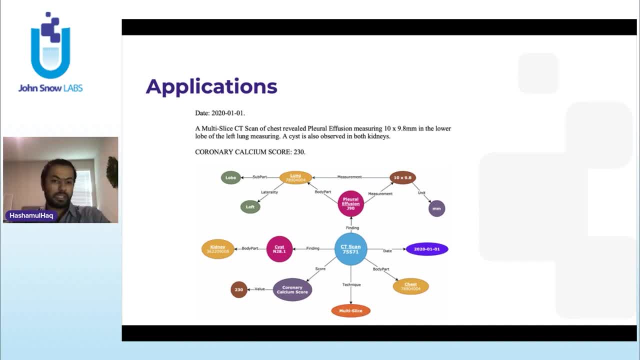 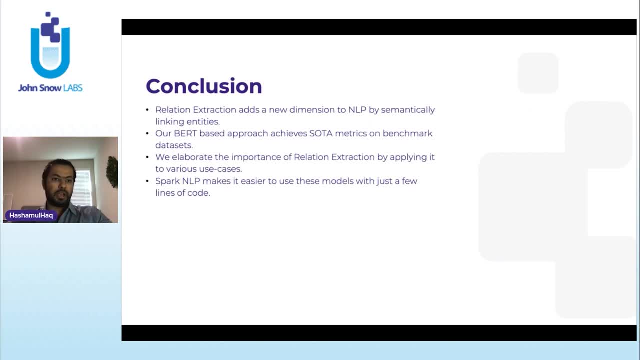 and feed that to the resolver model and get better results. So this is again one very cool and useful application of relations, And now we'll see how this, all of this, is actually. all of this actually happens in the form of code because we've made it easier to. 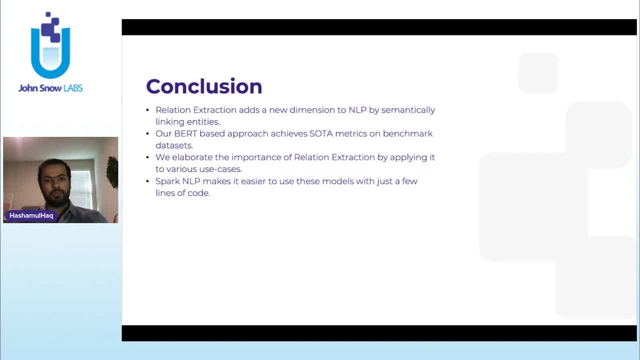 this sounds a bit scary, but we've made it easier to use these models. You just need to run a couple of lines of code. I'll show you. you can even do it in like 10, three lines. So let's go to the coding section. 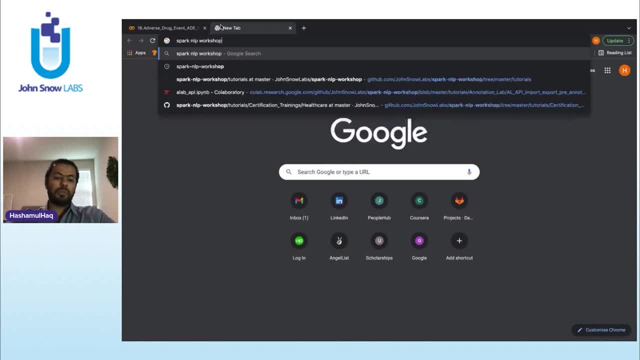 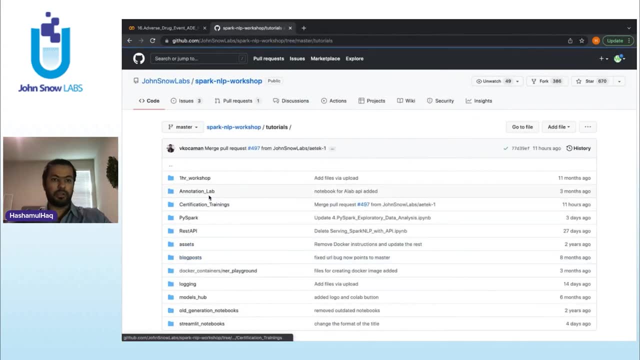 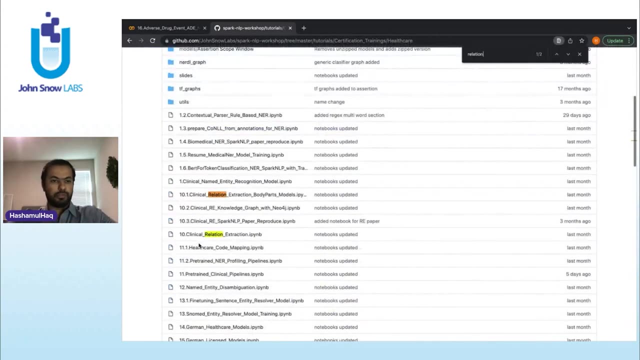 By the way, these are all these notebooks that, the notebook that I'm running. all of these notebooks are available here: Spike, NLP, Workshop, Healthcare, All of these notebooks are here. If you go here and search for relations, you would find a bunch of relation extraction notebooks. 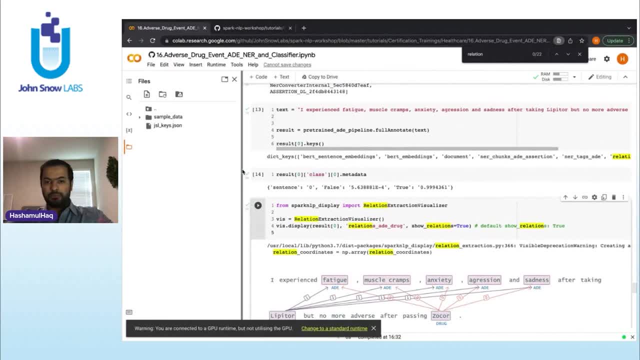 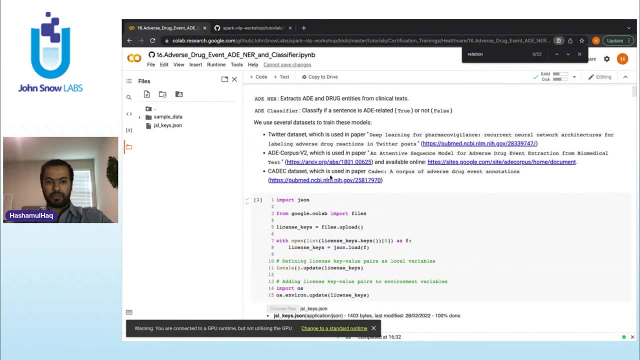 And, And. you just need to get started. You just need trial license. You can go here, open up any notebook, run the first cell, upload your JSON key and the next cell. it would install and get the setup ready for you. 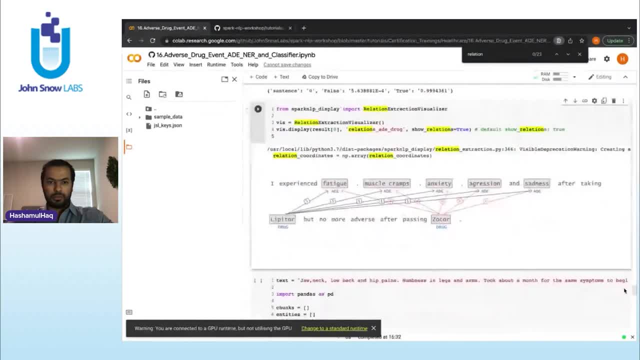 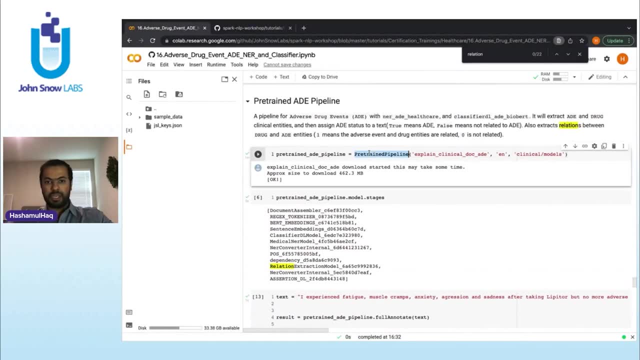 And then you can start exploring. But over here, if I show you how easy it is to use these models, you'd see that I have a pre-trained pipeline for adverse drug events- X-PlaneADE- And this pipeline contains NER models, assertion models, relation extraction models in a single pipeline. 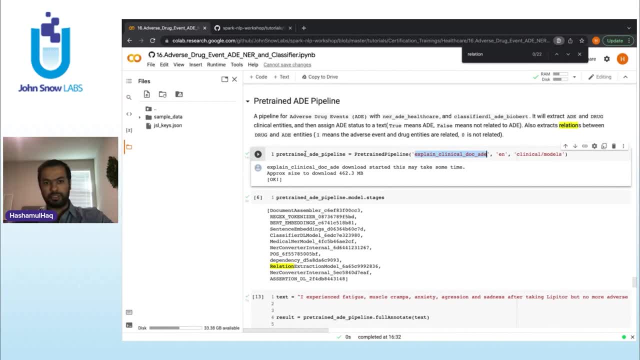 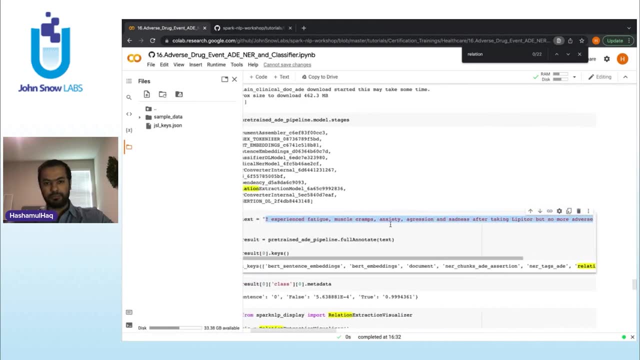 So you don't need to create a custom pipeline. You just write or you just execute This line of code. it would download and you can see the stages, and afterwards you just pass in your text. This is the text you pass in: do dot, full, annotate and it would give you the result. 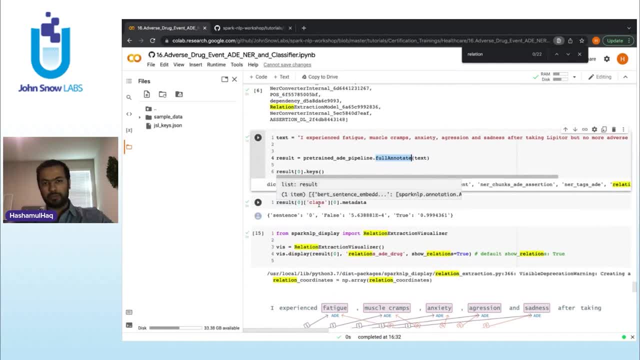 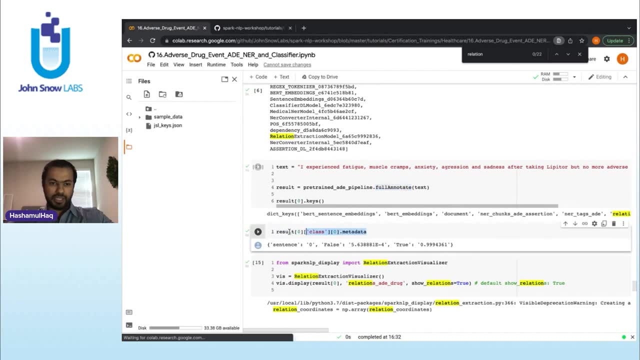 So in this we also have a classifier. This is a very elaborate pipeline. We have classifier models, like I said, NERs, et cetera, So I can check the results of each and every stage. So, for example, if I say I want to see 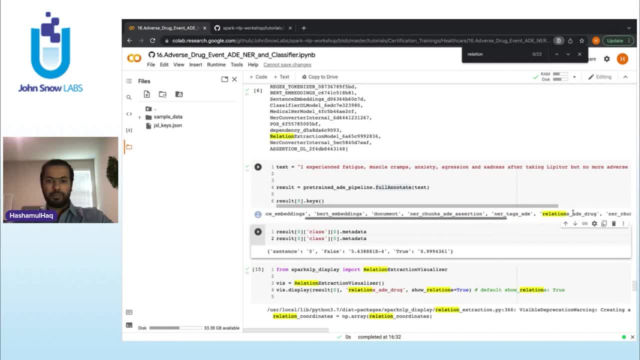 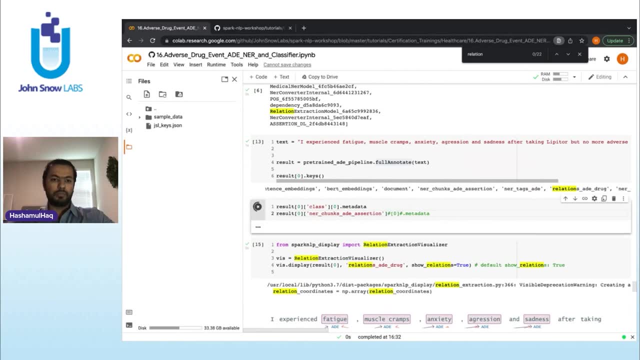 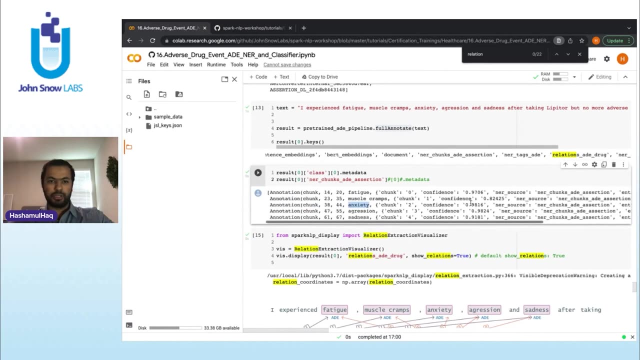 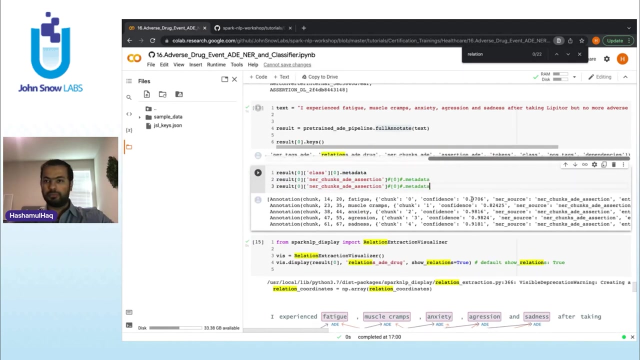 Result of, Let's say, NER chunks. Yeah, I can get chunks right. The P, the type is ADE, So these are the chunks, And if I want to look at the relations, I would just do This: 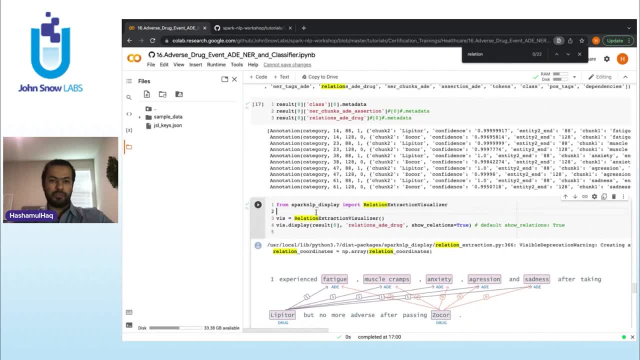 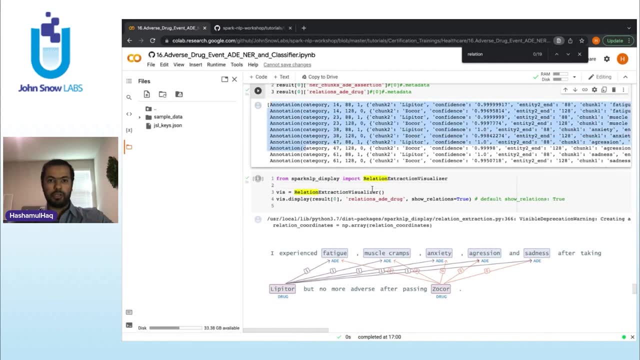 And this would give me, And we also have a display library which basically makes it easy for you to, because this is a data frame that you need to parse. So if you don't want to do that and want to iterate over quickly, you can just use a visualizer. 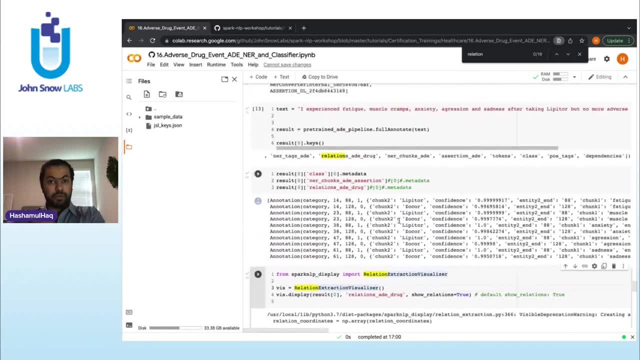 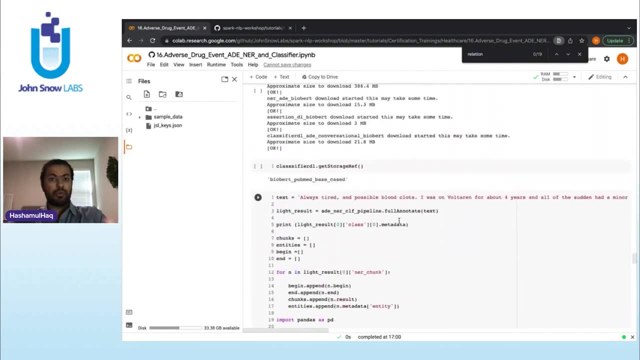 It would visualize things for you. This is a pre-trained pipeline that, as you can see, is just less than 10 lines of code, But if you want to create your own pipeline, you know, like I showed you, we have 10 different models. 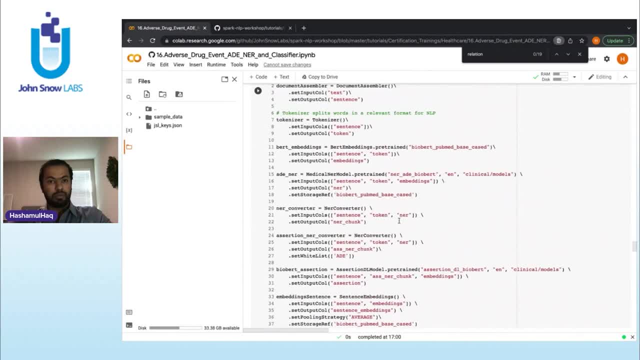 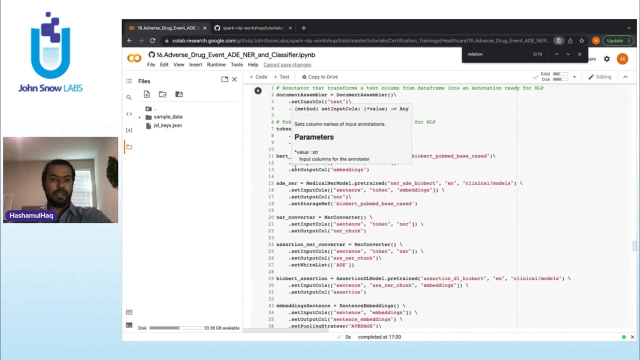 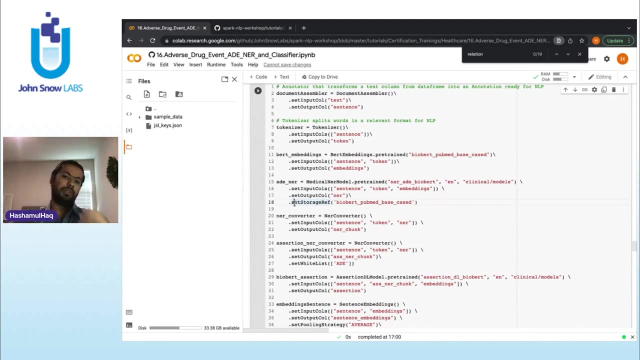 If you want to play with different models and see how does that work, you can write like this piece of code. We have trainings available for this as well. But the idea behind this is you run a basic NER model. You get dependency structure of the document. We use this dependency structure to basically filter out relation pairs. 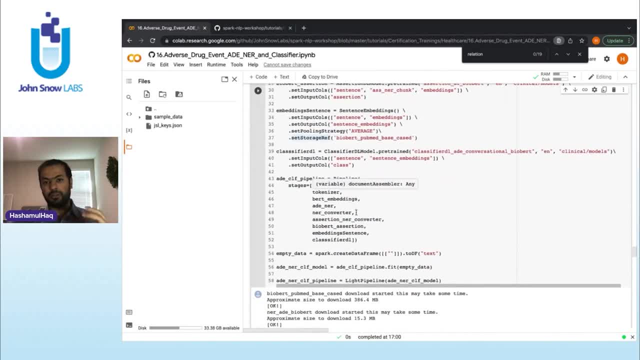 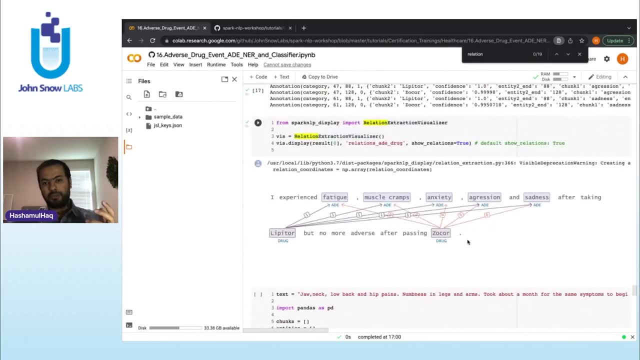 Not only relation pairs but, like you know, probable or candidate relation pairs, because if I have too many, for example, in this example we only have two different drugs and four different ADEs, But if in an example, if there were many drugs and many ADEs, it would explode exponentially very quickly. 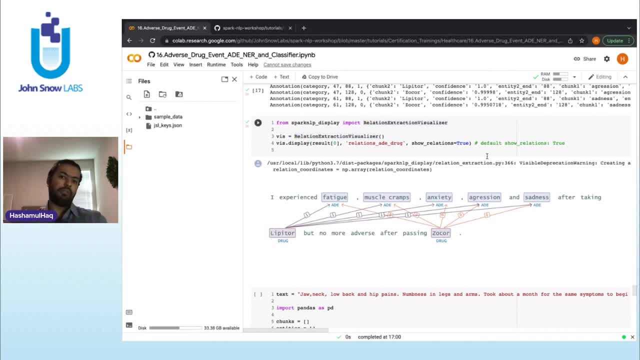 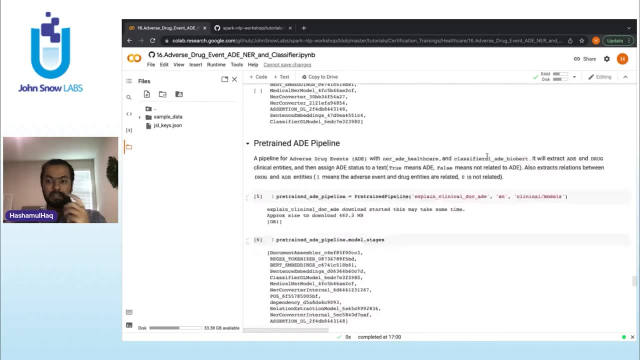 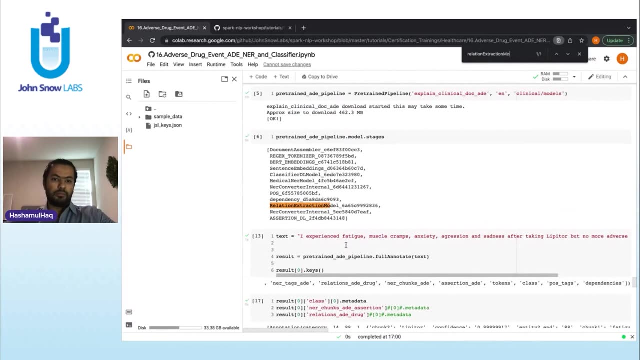 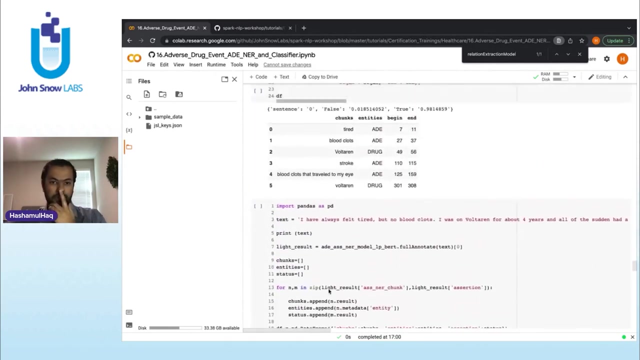 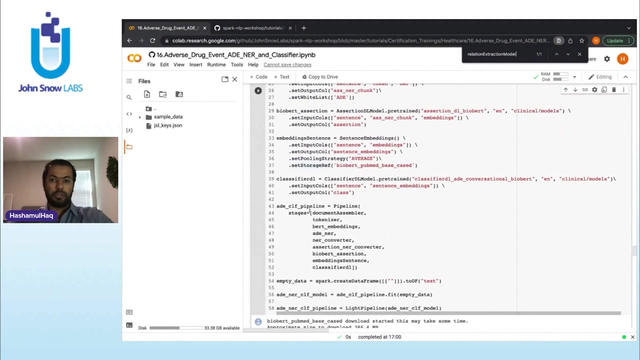 So we use dependency structure to basically reduce all that stuff down and only allow or only classify eligible pairs And this helps us on the computation cost. But this is how you can simply. You can simply load up or create a custom pipeline and create relation extraction pipelines and practice with it. 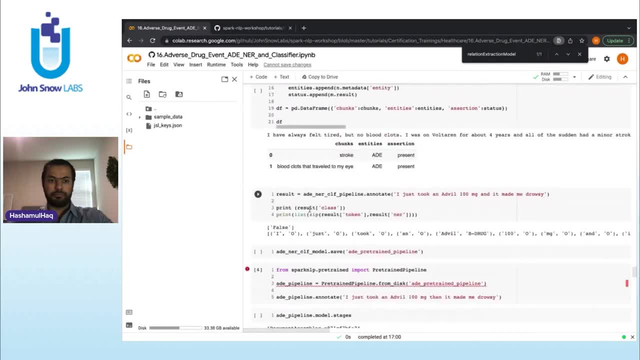 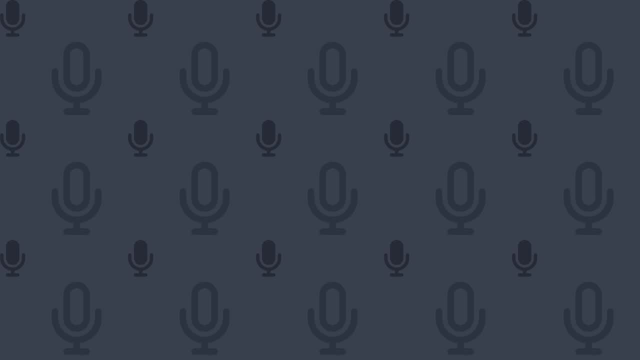